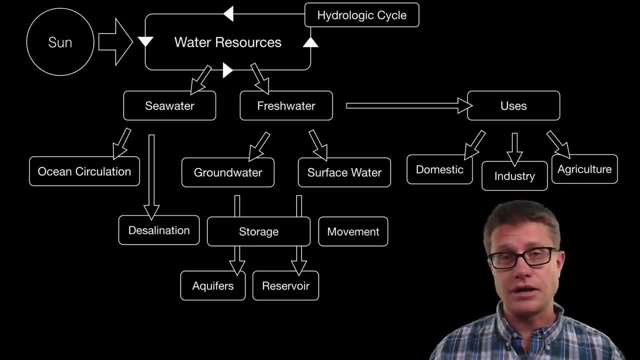 What about the surface water? Well, it can be stored in reservoirs that occur naturally, or ones that are created as we produce dams, And then we can move it around through aqueducts and even to the planet itself through irrigation. But we have a finite amount, And so conservation. 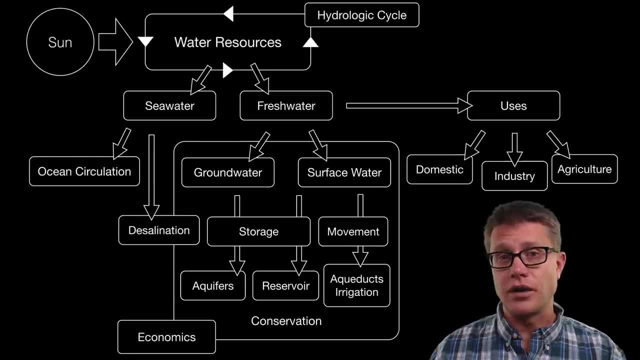 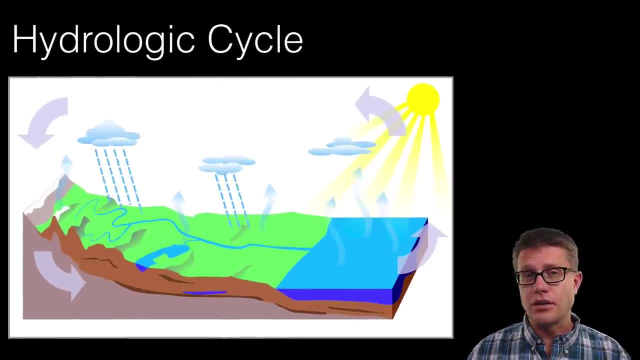 is incredibly important, And economics have contributed to water loss and could help us to actually solve this water conservation problem. And so the hydrologic cycle works like this: Anywhere there is water on the surface, we can have evaporation- I have so evaporation That gets cooled and eventually leads to condensation and precipitation Once 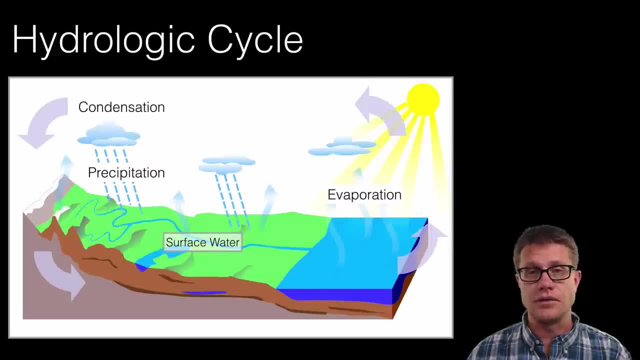 it is on the surface. we call that surface water. It is running over the surface. That could be lakes and swamps and rivers. After we have that water hit the ground, it can, however, be infiltrated into the soil and the ground itself. To give you an example of that, imagine: 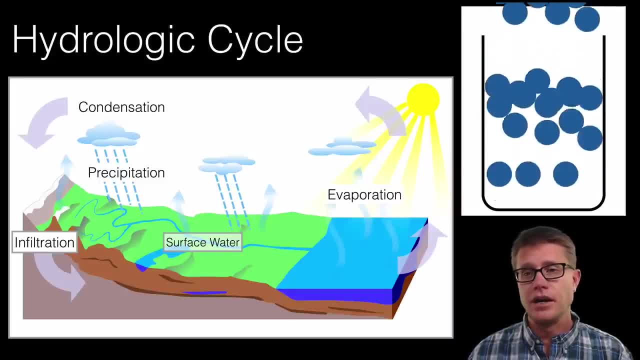 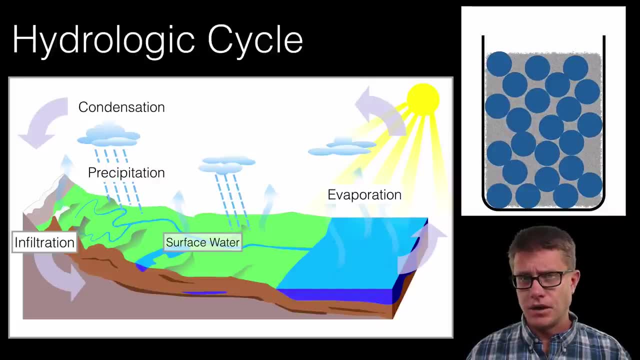 I have got a beaker here. Is it full? Well, maybe full of air If I put marbles in it. is it full? No, You can see there are spaces in it. What if I fill it up with sand? Is it full? No, There are still spaces in there. If I fill it up with water? now we are starting. 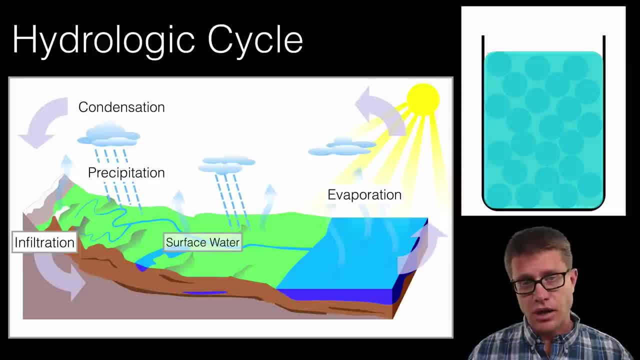 to fill up that beaker, And that is what infiltration is. As the water flows down into the soil, we call that now ground water. Let's say it is not filling that whole beaker. It is right here. That point at which we have saturation in the ground water is called the water table. 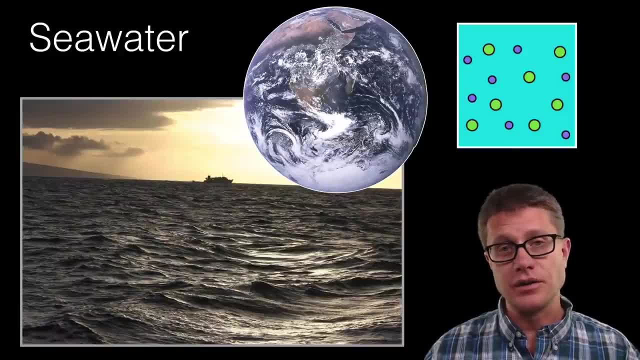 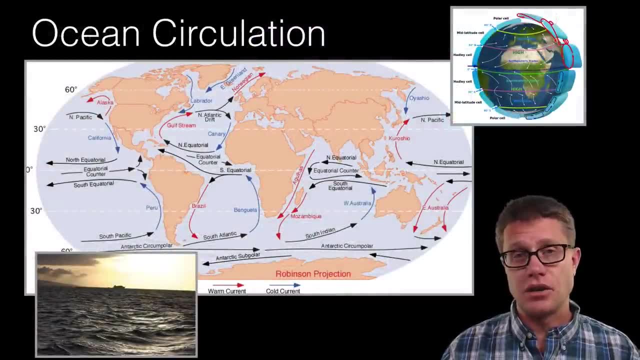 Most of our planet is covered with water. Unfortunately, it is sea water. It has salt dissolved in it. If you drink it, you will die. If we put it on our fields, the crops are going to die. It moves around using currents. We talked about that in the last video on the atmosphere. 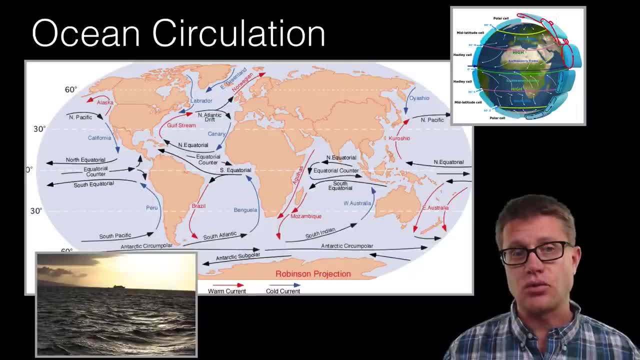 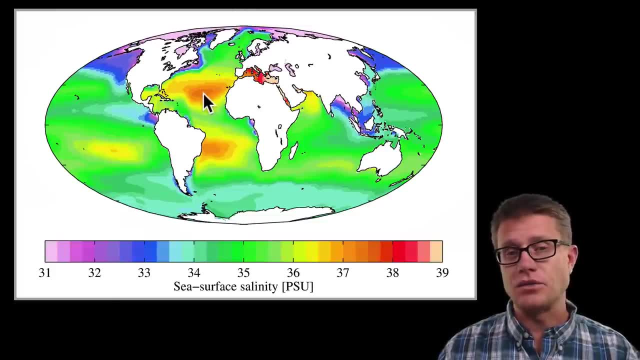 It cells in the atmosphere and the Coriolis effect. So we have these general trends in circulation. But also salinity affects it And so if we look at an area right here, it is a high salt concentration because we have a lot of evaporation, But up here we have 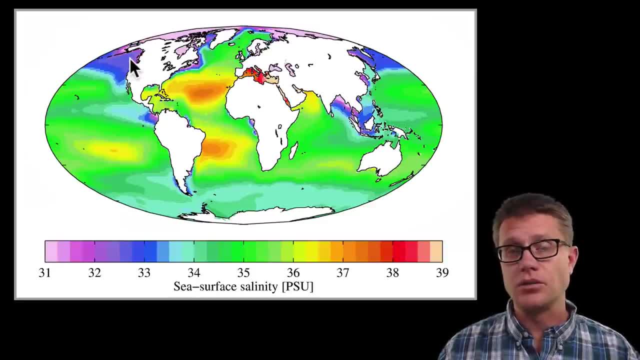 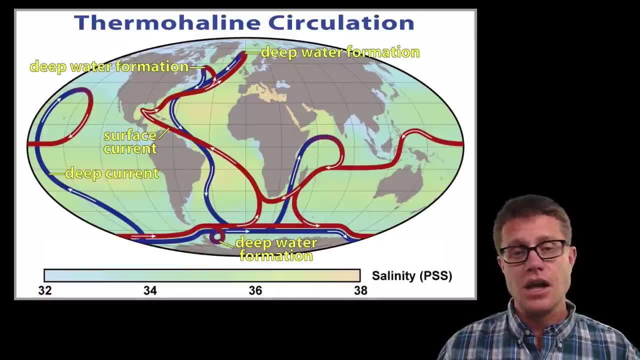 a lot of melting of that glacial ice, and so we are going to have a low salt concentration, And so the salt concentration and differences in heat create these thermohaline circulation and really make that whole ocean on our planet one system. Now, if we look at fresh water, 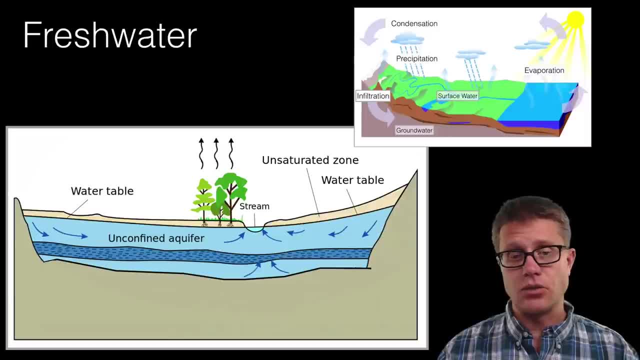 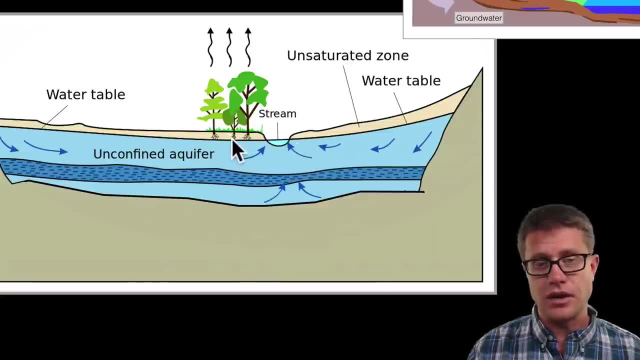 it can be divided into water that is above the surface. We call that surface water And then ground water. But what is interesting is if we look to the sides of that stream you can see the water table in the ground water. And so if you dig a hole right here, 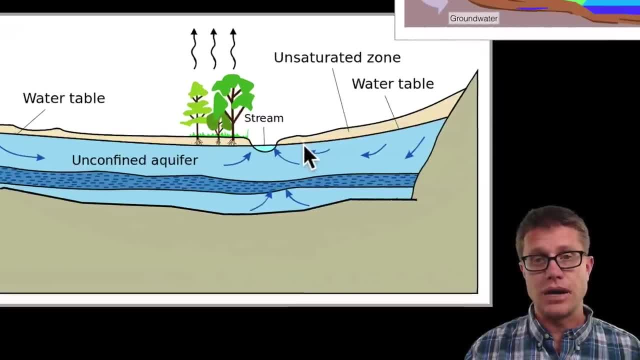 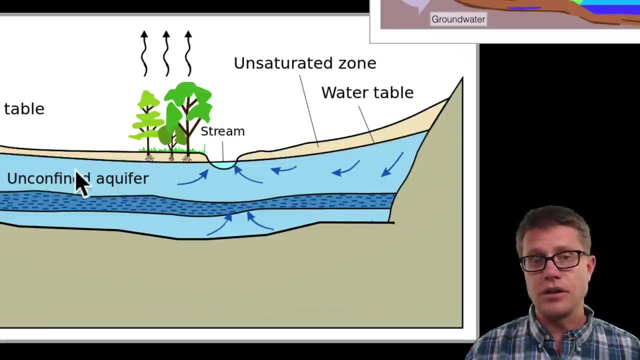 it is just going to fill in with water because of all that ground water around it. Now, this is an aquifer. It is storage of that water in the ground water. We call this unconfined aquifer. Sometimes the water can move between the surface and the aquifer itself. If I were to dig down 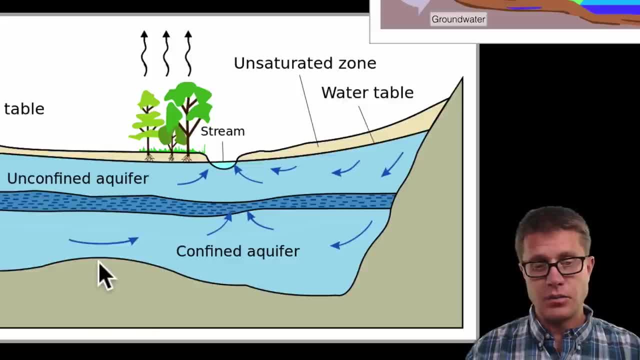 a little bit, we could find what is called a confined aquifer And that is going to be stuck between this impermeable rock down here and above it. Now let's say we want to get to that ground water on the surface. If we want some of the surface water, we simply pump. 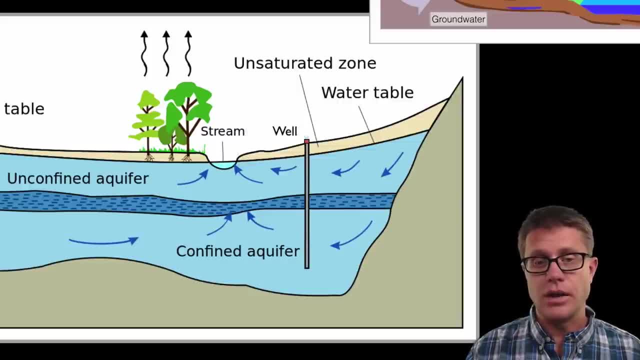 it out of the stream. But if we want to get out of that ground water, we could dig a well. Now the water, we could either pump out the water or sometimes we will have what is called an artesian well, Where there is either enough gravity above it or there is a lot of water. 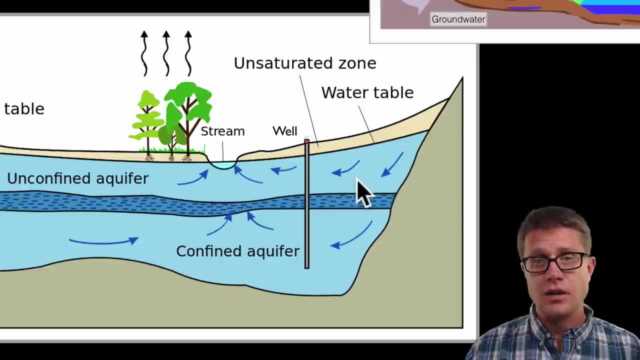 in it, or enough pressure in the ground water so it actually comes out. But as we use that- well, just like using a stream- the water table is going to drop, And so we are going to start to deplete that aquifer. Now, an important term in filling an aquifer is something called 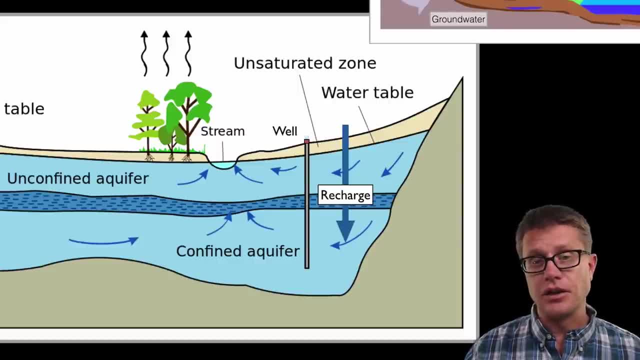 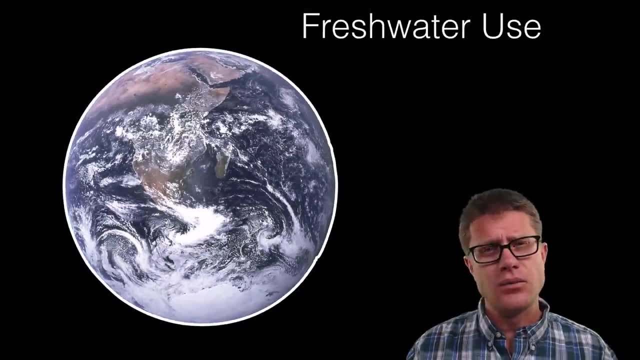 recharge. So as we get water and infiltration, we are going to fill up that aquifer. But if the outputs, in other words, if we pull out more water than we are putting in, we are going to deplete the aquifer. And what are we using all this fresh water for? Well, 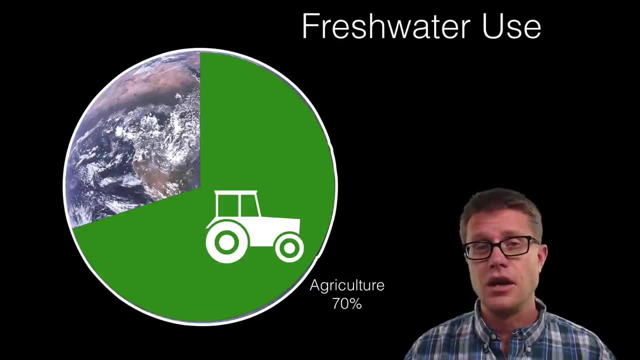 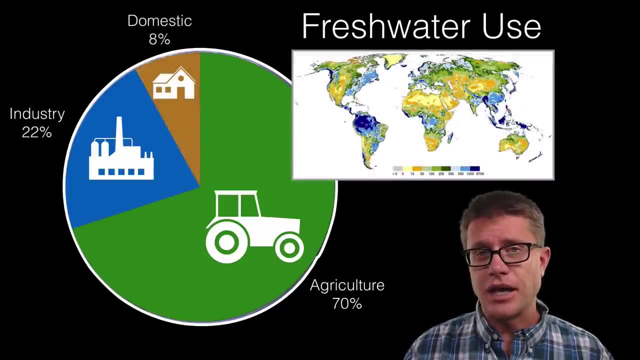 if we break it out using a pie chart, most of it is actually for agriculture. So we are going to use it for agriculture, The growing of our food. We use some of it for industry and then some of it domestically in the house. The problem again is that it is unevenly distributed. 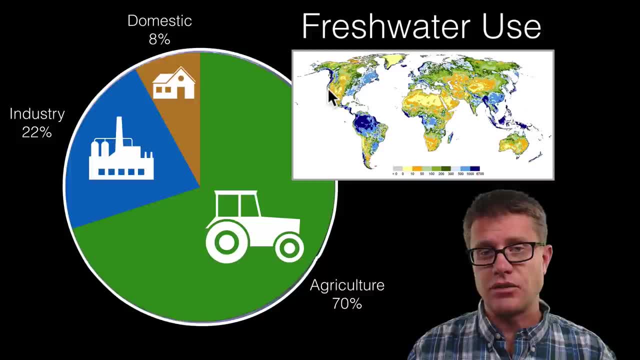 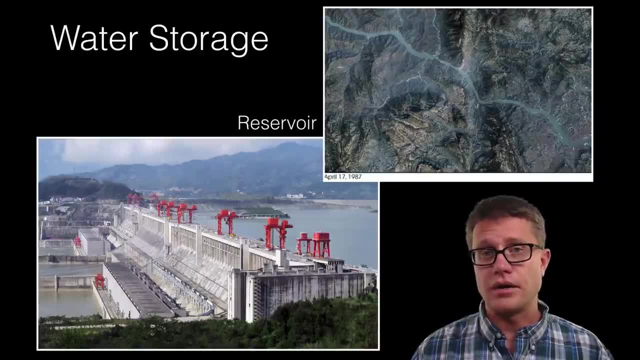 on our planet. Brazil is going to have plenty of water, but if we look in the desert southwest of the US or in the Sahara, there is not going to be any water right there. And so what have humans done? We have started to store water. So reservoirs are an example of that, A big 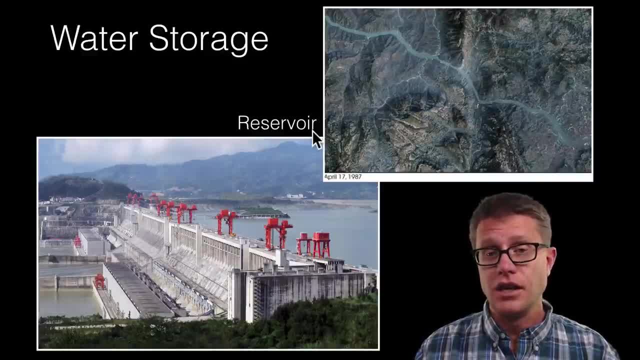 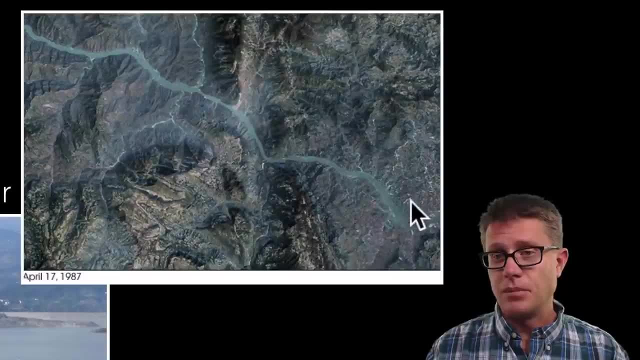 example would be the Three Gorges Dam that was built in China, finished in 2006.. And so this is what that river, the Yangtze River, looked like before they built the dam, And then they built the dam. It finished in 2006.. You can see what it looks like then. So we are storing the water behind. 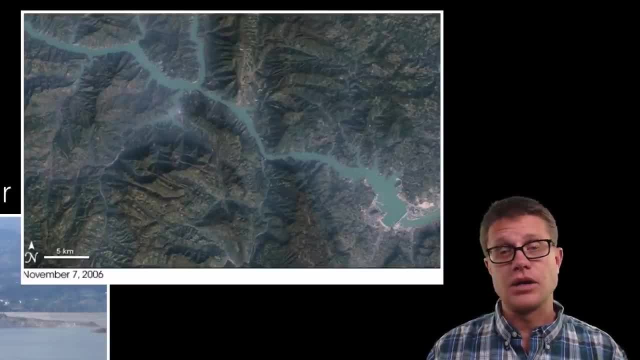 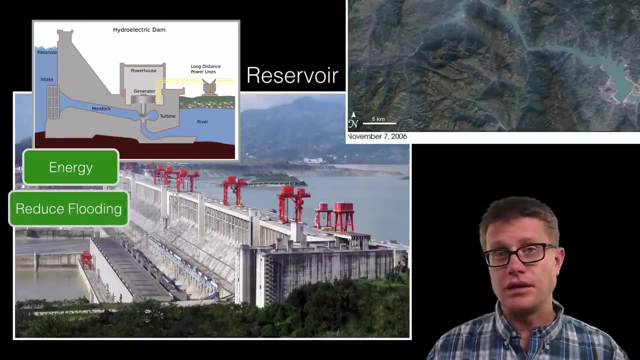 the dam. What is nice about that? Now we have water that we can use at will. We also can get energy from it. as we run that water through a generator, We can control flooding downstream, And also we can use that for irrigation or the Three Gorges Dam they are using to increase. 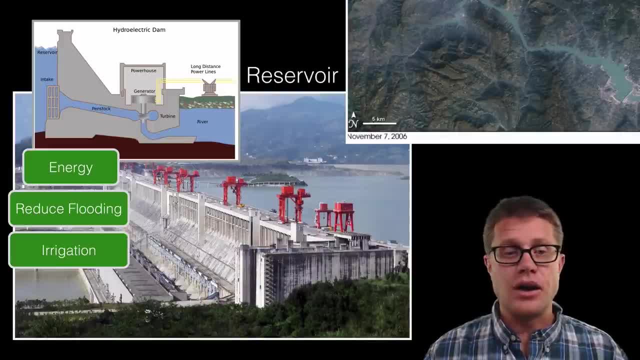 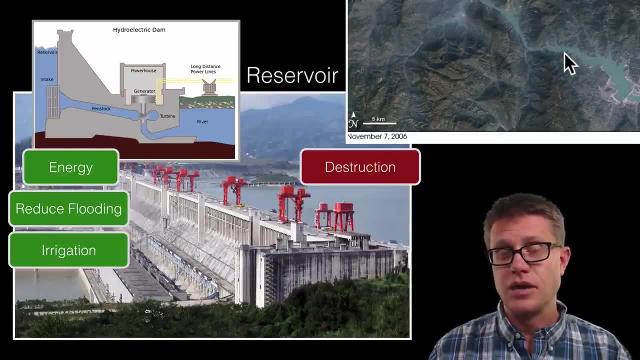 shipping on the Yangtze River. So it sounds great. What is the problem? Well, there is going to be destruction wherever that water went. So we are decreasing 20% of the forest in this Yangtze River. We are displacing over a million people that used. 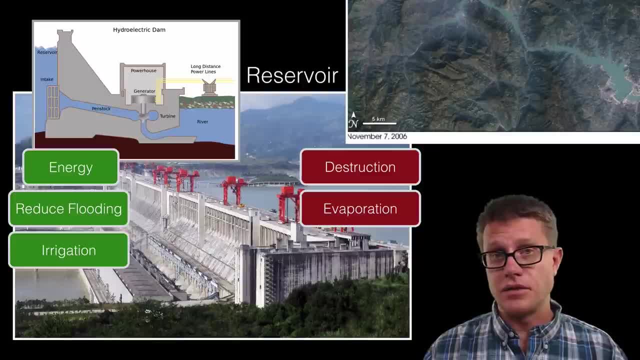 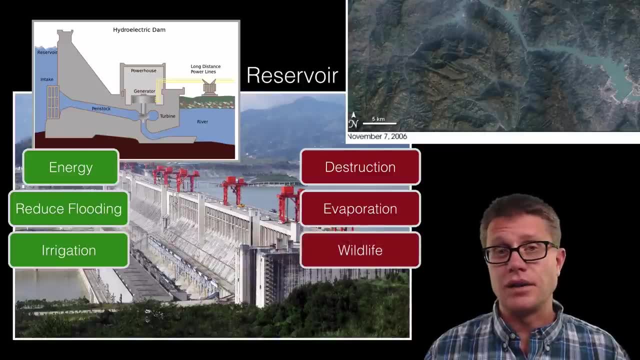 to live there. We also have evaporation of the water off the surface, And then we are going to have nutrients that start to deposit there that would have normally moved their way down the river, And that is going to disrupt wildlife, And so fish obviously cannot spawn. 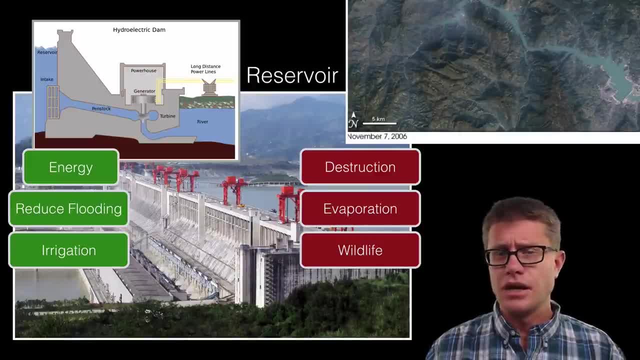 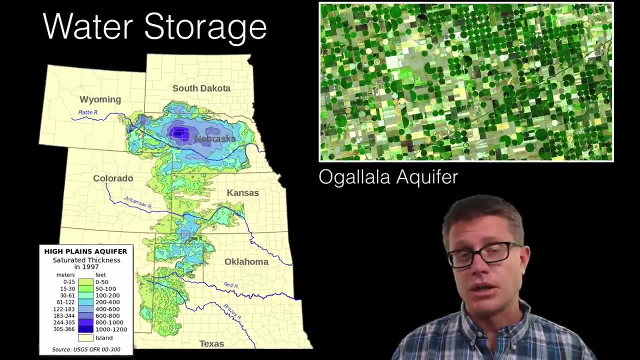 move up and down in the stream, But it is also going to change the temperature of the water. Example: there is a freshwater dolphin that went extinct in the Yangtze River And the Three Gorges Dam may have contributed to that. We can also store it underground. That is naturally stored in what are called aquifers. 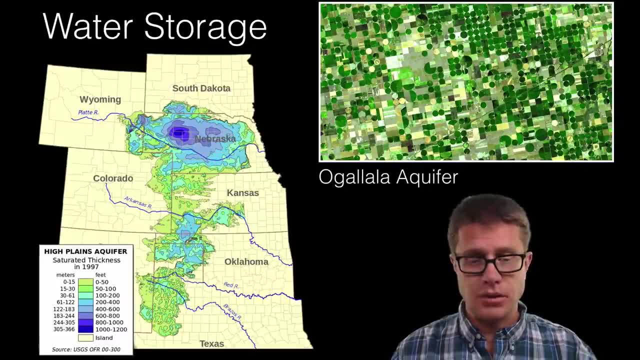 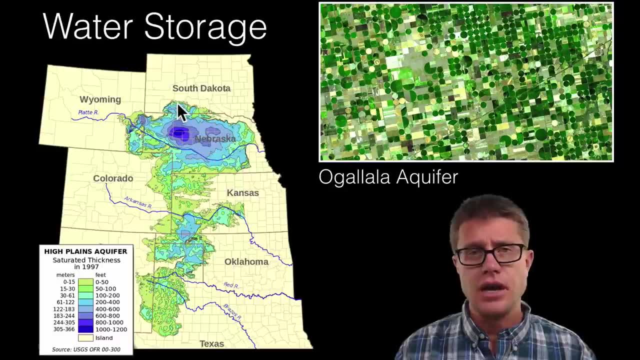 One of the largest ones on the planet is the Ogallala Aquifer. It is going to be found in the Midwest, And so here it is in Nebraska, But it goes all the way down to Texas and up into South Dakota. It is a huge aquifer. So if we look at the amount of water stored, 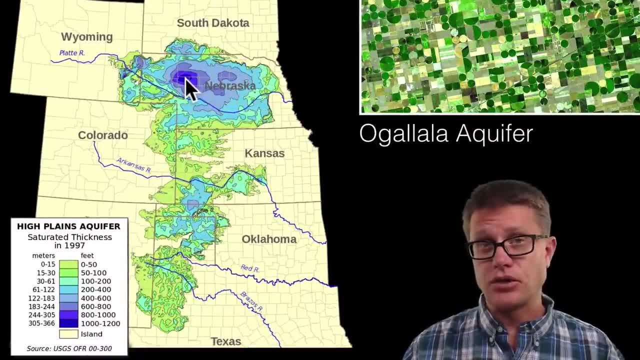 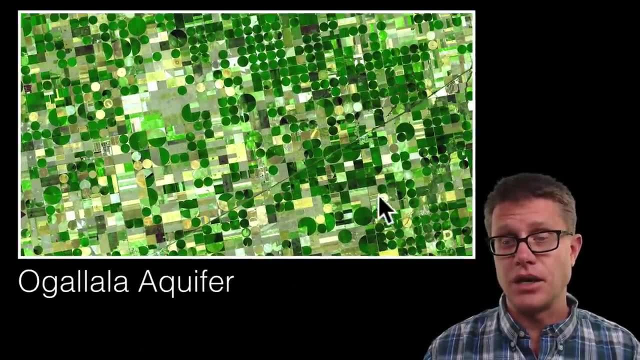 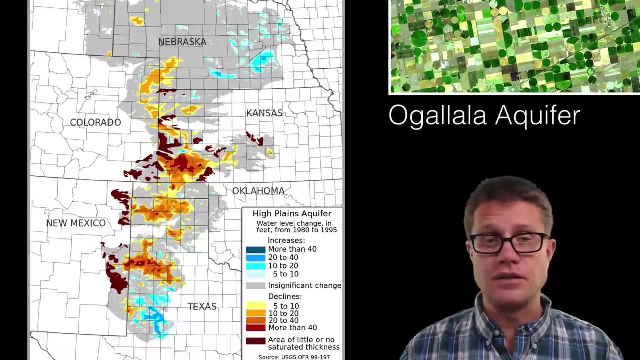 underground. it is over 1000 feet of infiltrated saturated water underneath the ground that we can use. You can see right here there is tons of irrigation going on. This is in Kansas. They are using center pivot irrigation so they can grow their crops. It seems great, But what happens again? 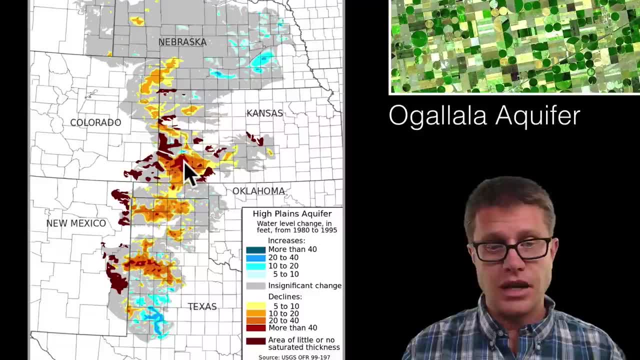 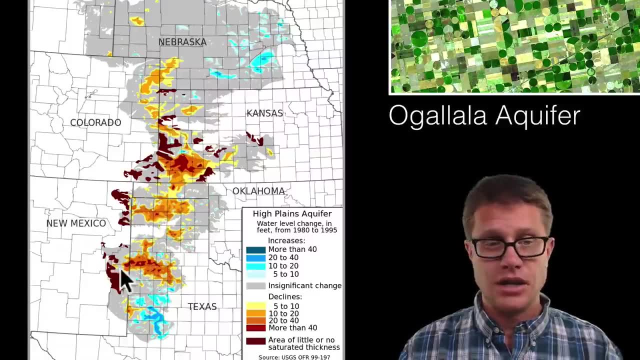 is that we can deplete that. So if we look at, this is during a 15 year period of time, There is an increase in the aquifer in certain areas, But most of the time we are seeing depletion And sometimes that aquifer has kind of disappeared. And a lot of scientists 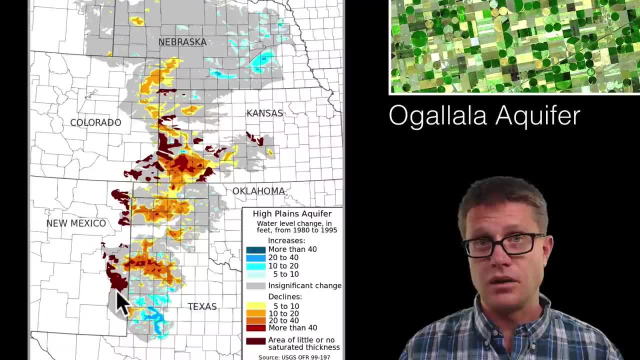 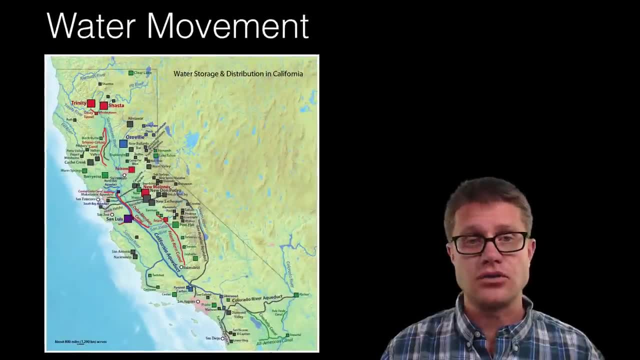 think in the next 100 years the Ogallala Aquifer is just going to disappear. Why is that a problem? Because it is going to take another 6000 years to fill it up again through recharge- natural recharge. Now we also have to move water around, So looking to California is a great example. 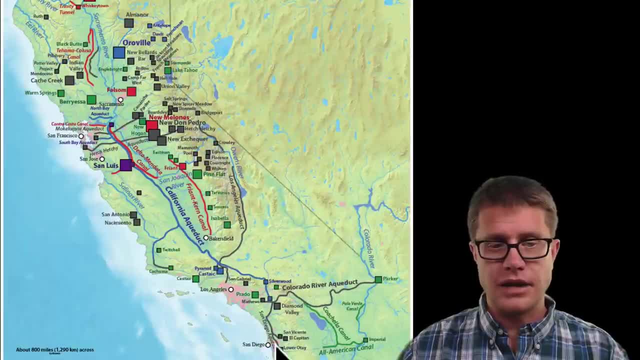 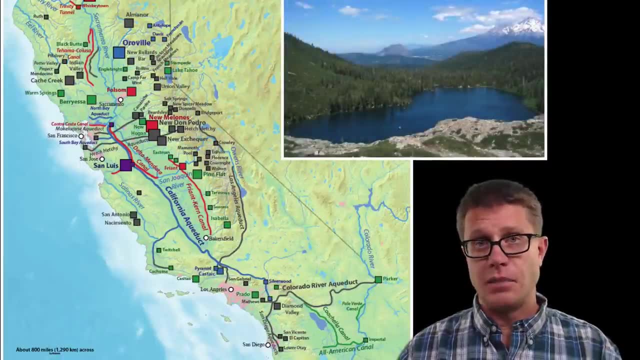 of that. So if we look in California, they need a lot of water in the Central Valley And then in the South Los Angeles and San Diego. So they built this huge system where they can move water where it is in the mountains And they can move it through these aqueducts. 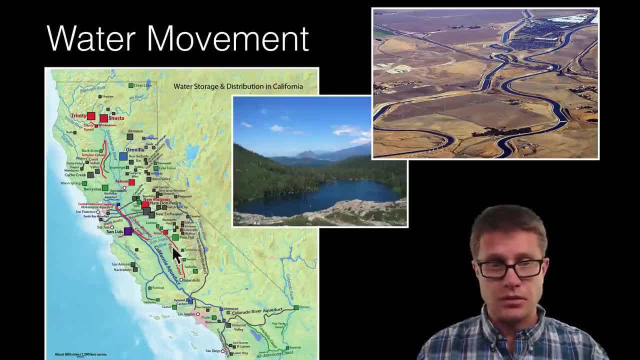 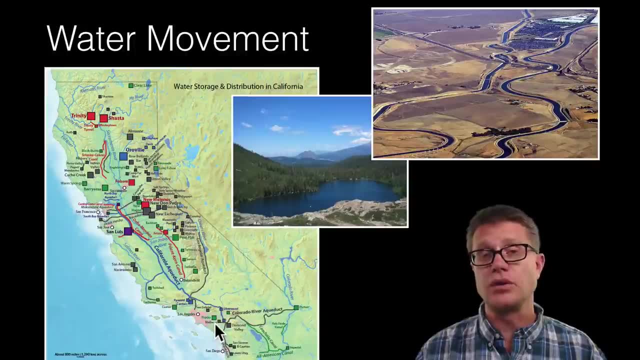 to where it is needed. Now you can see that is controversial. So people in this area are saying: you are depleting our rivers In this area. you are depleting our rivers In this area. we are saying: we have more population, We are growing your food, so we need more of. 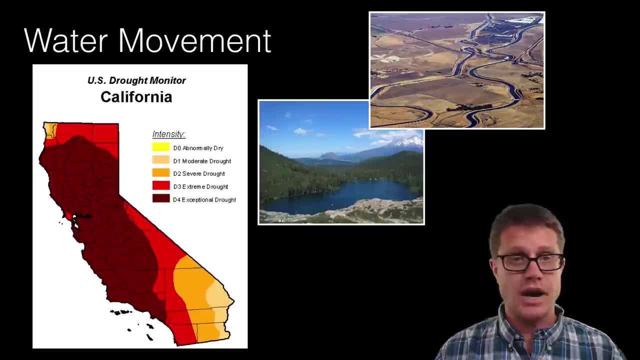 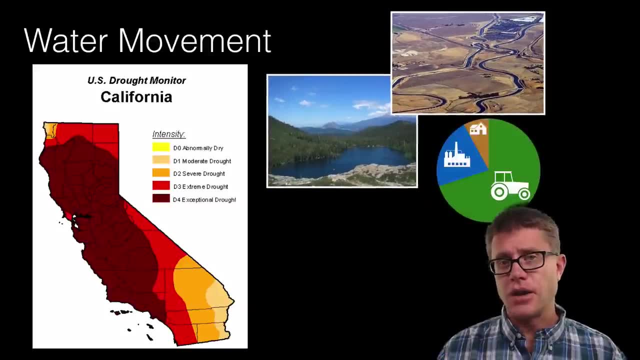 that water, And this conversation becomes more heightened when we move into drought, And California is in an awful drought right now. Drought occurs when you receive way less than the normal amount of water, And so, as we use that for agriculture, irrigation movement, 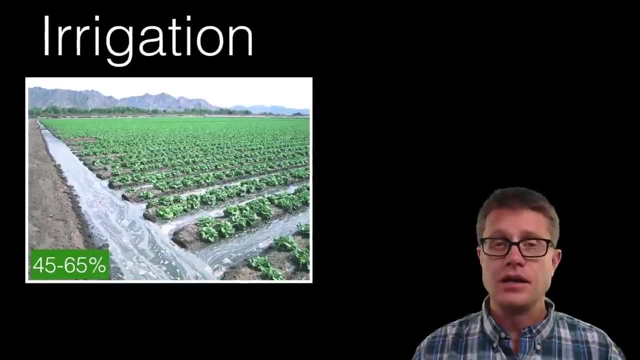 is super important. So how do we move the water actually to the plant? The easiest way to do that is using furrow irrigation. You can see it is easy. You just dig a trench. What is the problem? You have efficiency rates of around 60 percent. What is that? It is how much of the water. 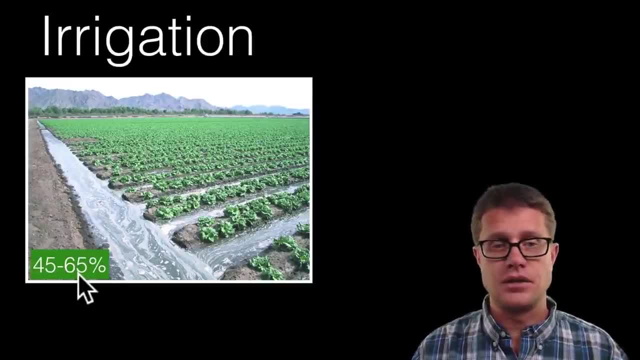 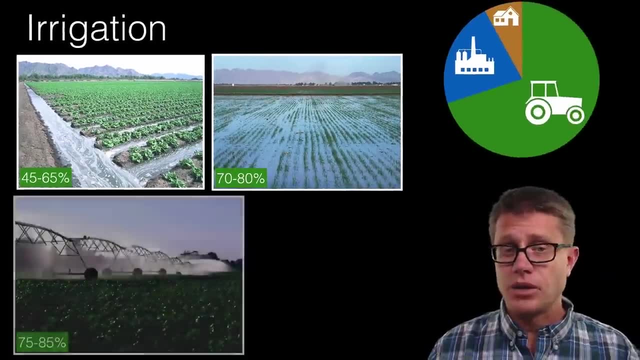 is actually going to the plant without being evaporated and infiltrated into the soil. So we could move to flood irrigation- higher efficiency- but it is going to damage the plant a lot of the time. We could move towards a spray irrigation- high efficiency- but what? 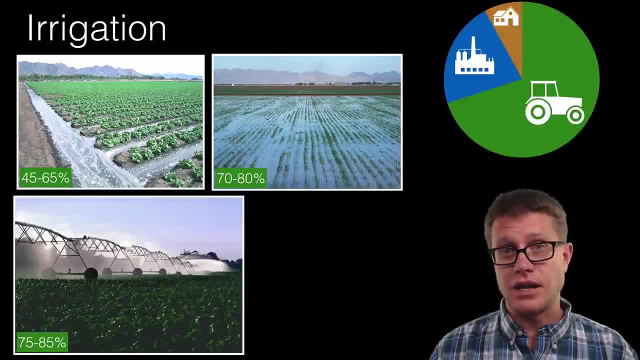 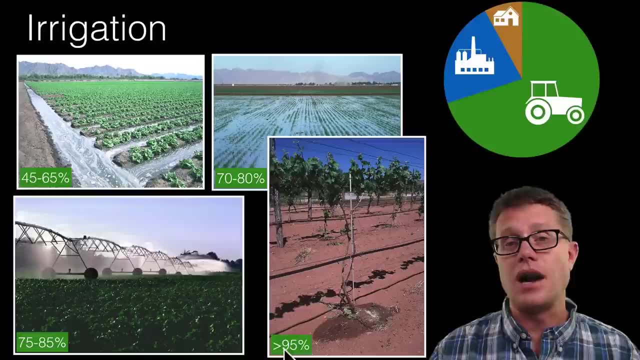 are we doing? You can see we are adding equipment. This is a center pivot, So that costs money. Or we could move to drip irrigation. You can see it is going to be 95 percent efficient but it is going to cost the farmer a lot more money to do that kind of irrigation And it 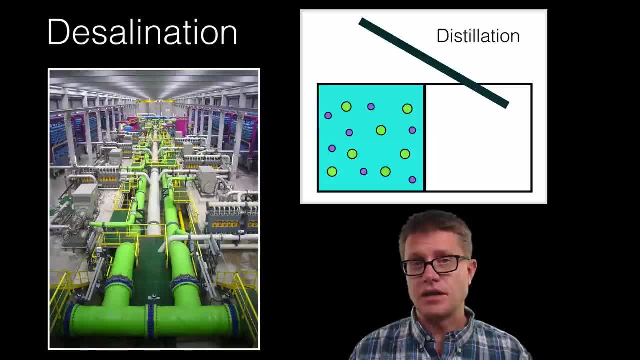 is going to cost a lot more money to do that kind of irrigation. As we move into drought situations, desalination becomes an option. We can remove the water from seawater. One way to do this is through distillation. What you do is you heat up the water and it. 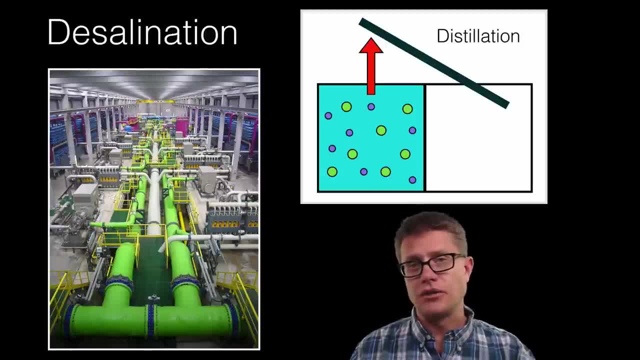 evaporates. It is kind of like the hydrologic cycle. You then cool it down, usually through pipes, And what you do is you remove the water. What is the problem? It costs a huge amount of money. We could also do that through reverse osmosis. This is a reverse osmosis plant over 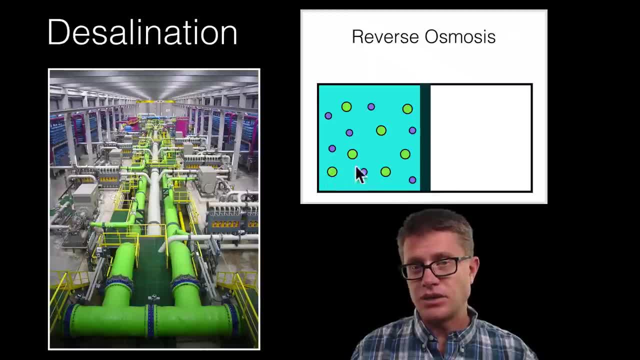 on the side. What you do is you put a membrane right here And then we squeeze the water. And as you squeeze the water, you move the water through, but you leave the salts behind. Now we have fresh water. What is the problem? It costs a lot. 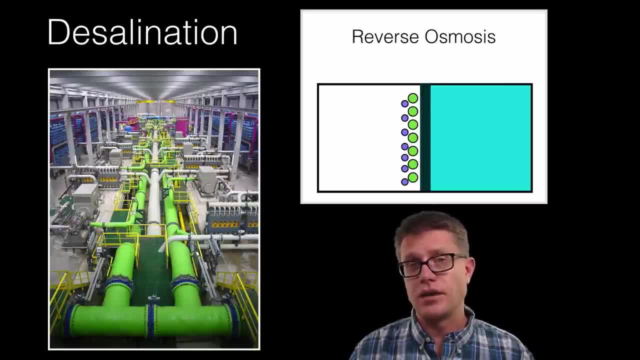 of money. About 1 percent of the people on our planet are using water that is created through desalination, But by 2025, we should have 14 percent of the people on our planet in water scarcity, And so desalination may be an issue.